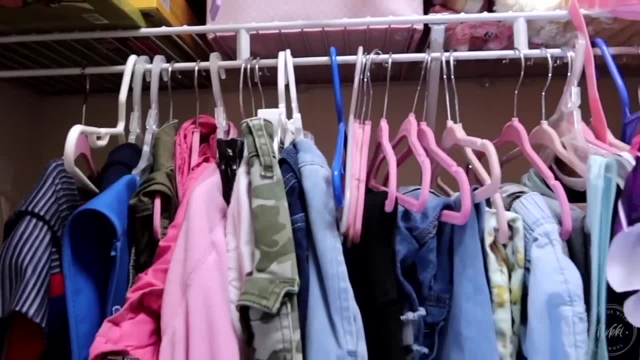 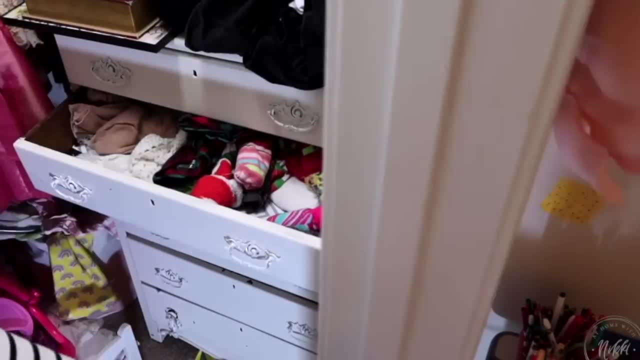 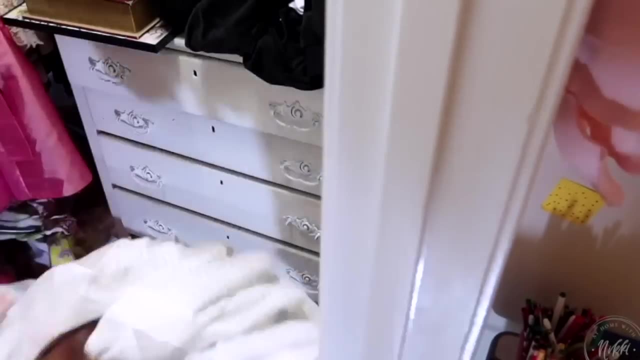 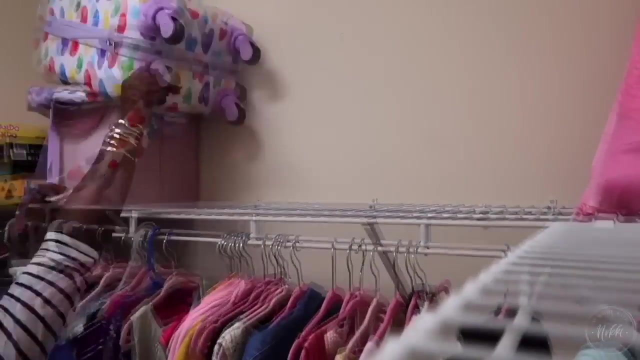 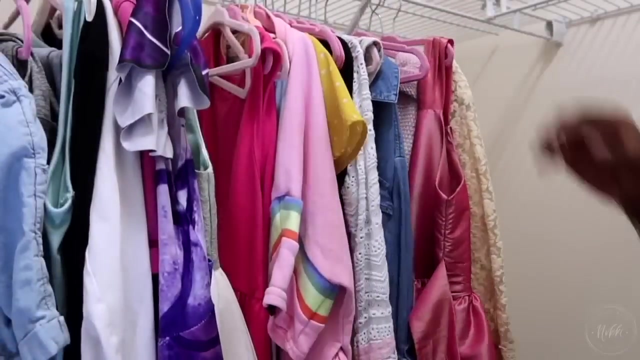 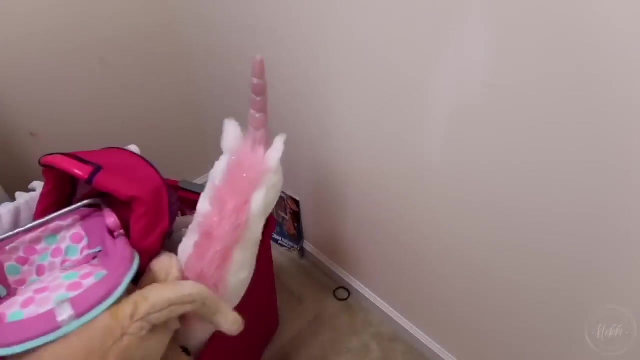 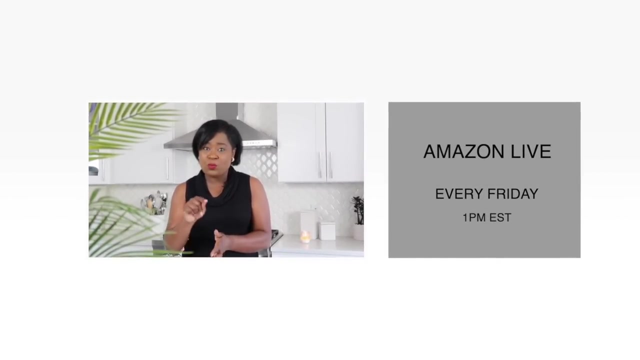 We're going to start by taking out of this closet so that we can categorize, downsize and then rebuild this into a beautiful space. Friends, I want to take a pause in the middle of this video really quick to let you know that I'm live on Amazon every Friday at 1 pm Eastern Standard Time. We have a lot of fun over. 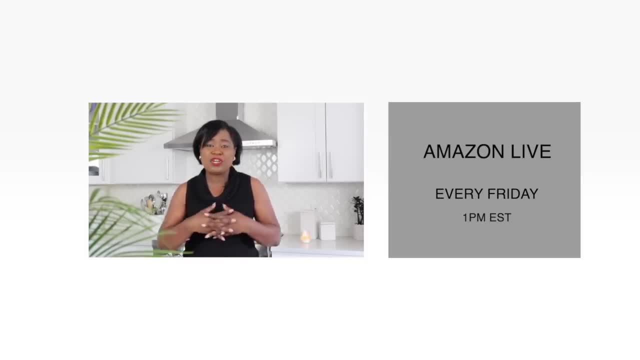 there We call ourselves the Friend Girls. We do things from sharing. I share a lot of Amazon products. We chit chat, We catch up. It's kind of our lunchtime, So I hope to see you every Friday, 1 pm, Eastern Standard Time. I'll see you there. Bye. 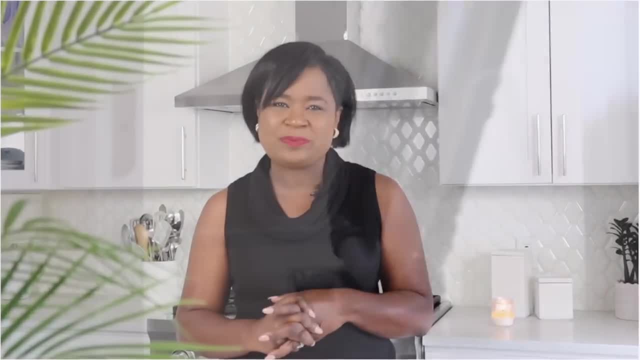 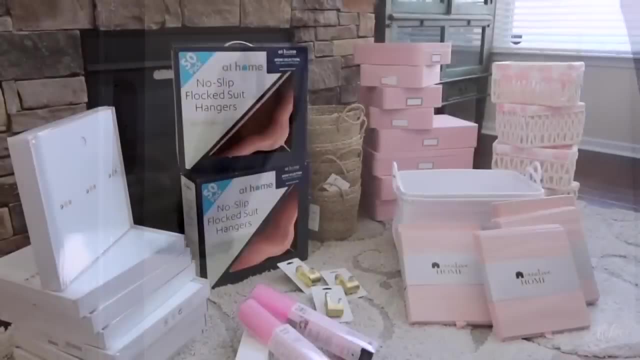 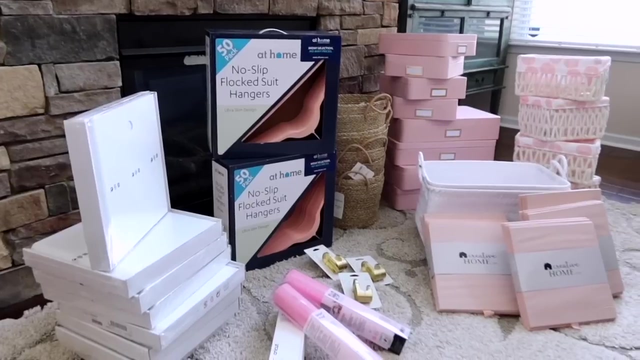 So, now that we have everything taken out of the closet, because I want to give myself a blank canvas to reset her closet, And so I went to a variety of stores- I actually went to At Home, Target and Ikea to get all of the essentials that I needed to kind of redo her. 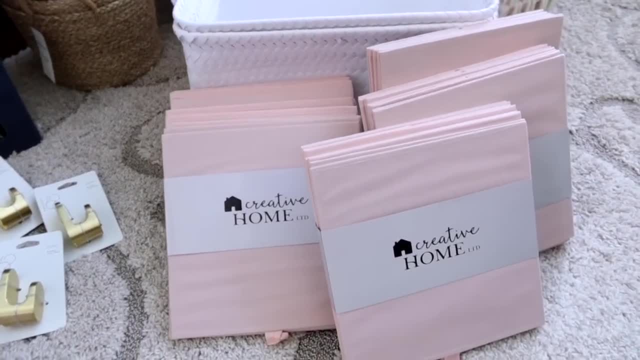 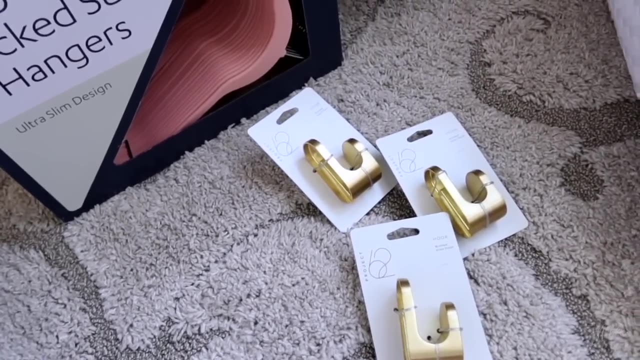 closet. I knew I wanted to go with these standard linen bins for the top of her closet because it really helps maximize space. I found these gorgeous gold hooks at Target. They're great for hanging things like book bags and coats and all of her purses and things like that. 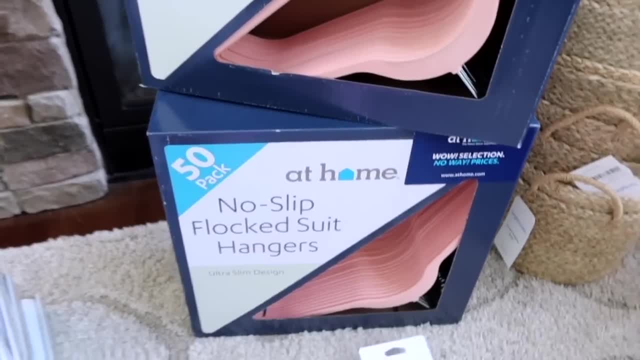 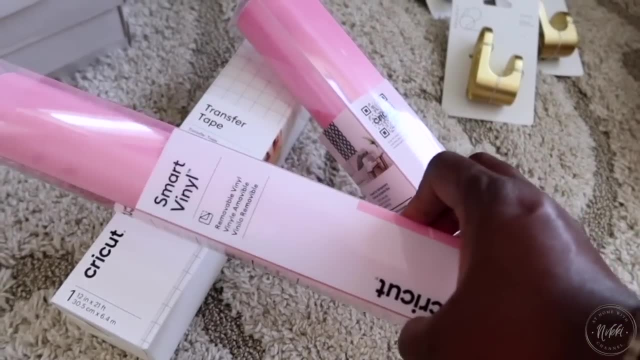 Also, she had kid hangers And now that she's at a bigger age her clothes really fit adult hangers, which makes it more efficient. along with these bins I got from Ikea and, of course, smart vinyl for labeling, And then I found these white bins in Target, which are going to be great for her games. 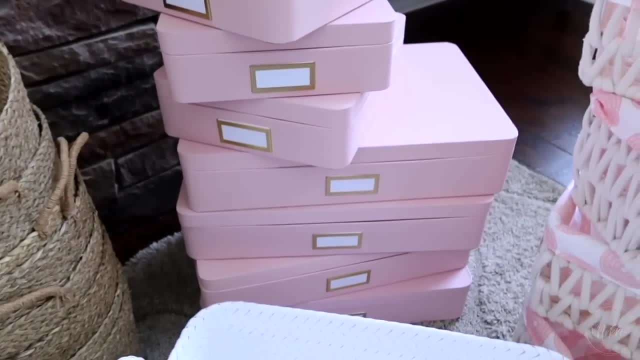 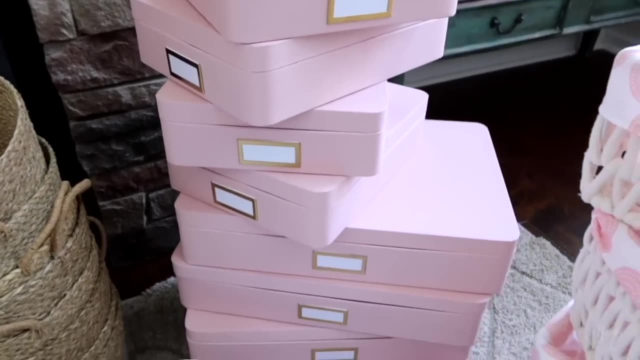 And then, of course, these nice little Target baskets that are lightweight and great for all of her accessories and shoes and things like that. And then these bins are going to be great for some of her puzzles and memorabilia and things like that. So it's important to think about how she works in the space And so 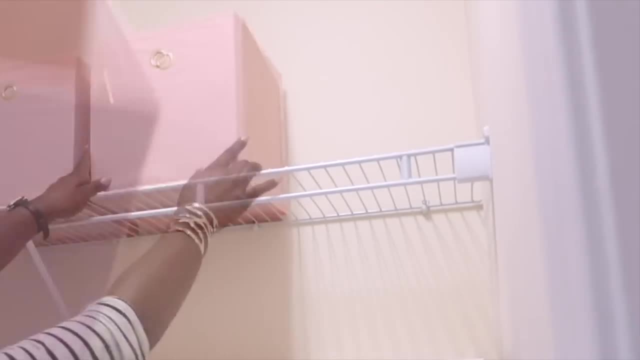 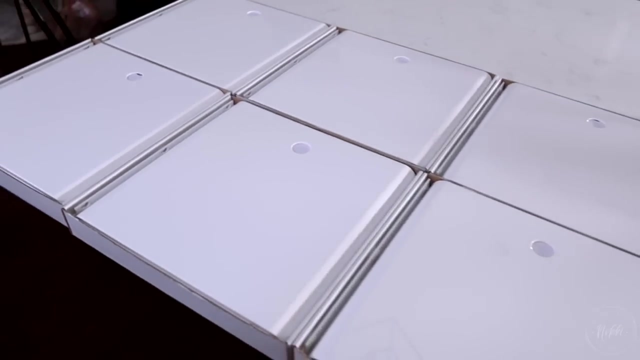 up top is going to be for her things that she doesn't really need, but more so her mom needs, And this is where we have some of her fabric memorabilia, blankets and things, her sheets for her bed and all of those items that her mom needs to grab. 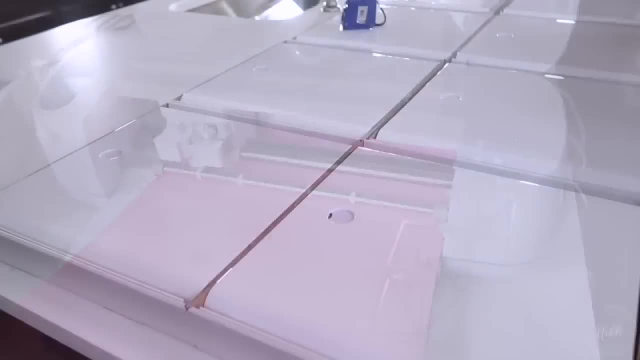 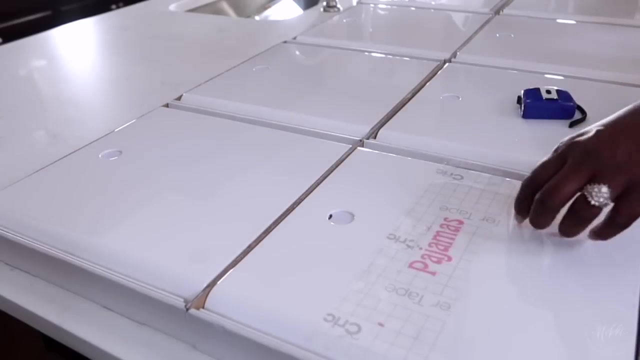 But Savannah doesn't necessarily need to grab Now. labeling is important because I am going with a bin system for her closet, which is great for a kid's closet, because it allows them the ability to be able to clearly see where their things go, how to put them back And when they do it. 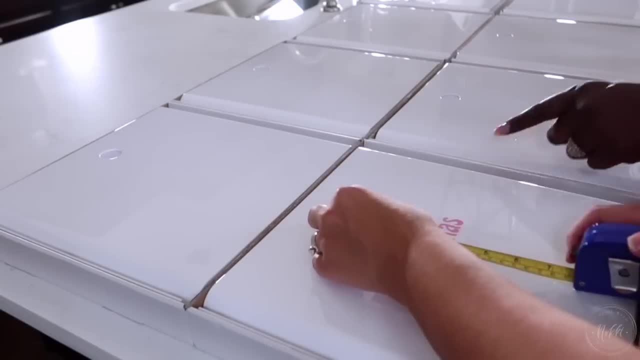 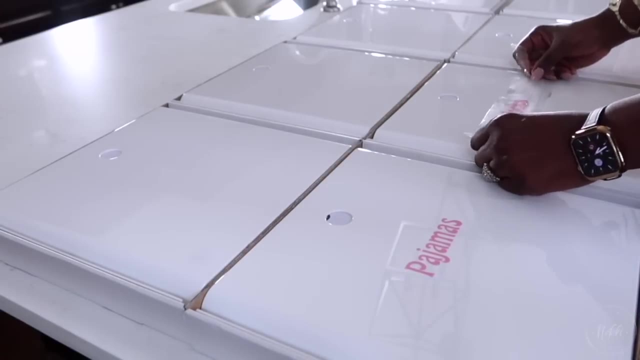 they don't necessarily have to fold everything neat or everything looks great, because you don't necessarily see the items, but they are at least categorized, which is really huge. Then, when they become teenagers, when you use the bin system, it's really easy to. 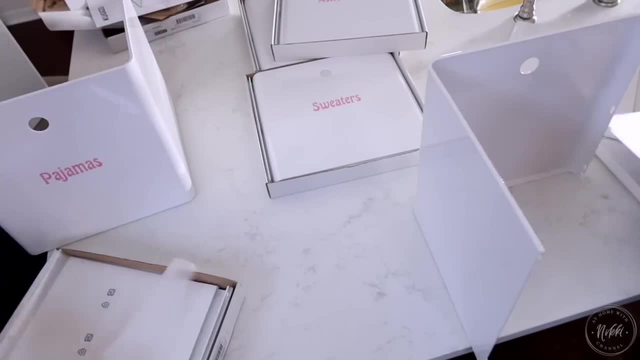 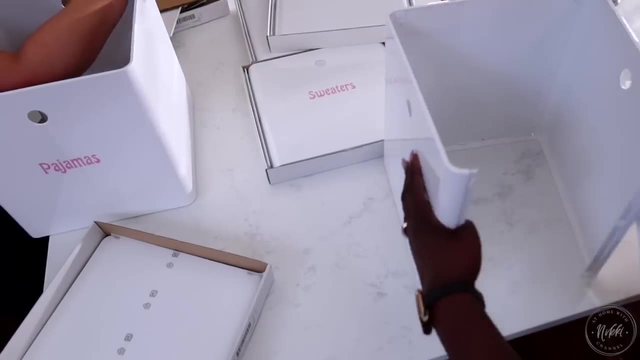 refer the closet back to just a standard closet when they no longer go with the bins, And so these bins are really sturdy, They're from Ikea and we want something that's really going to last for the kids. There's a lot of different bin options on the market, So you really want to be. 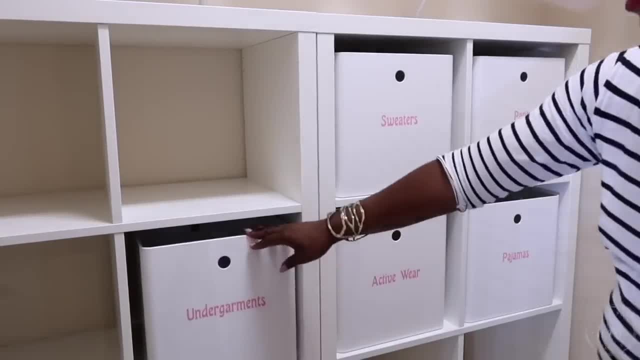 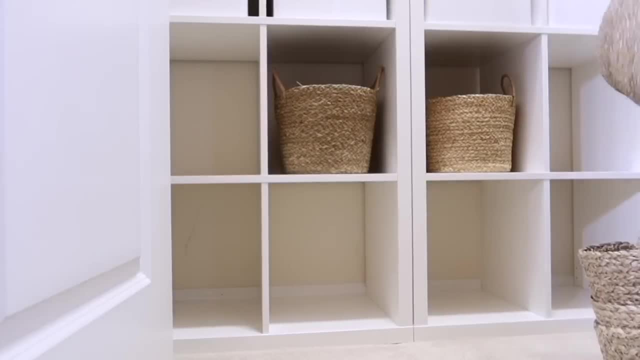 sure to go with something that really is going to hold up with the kid kind of handling it. Also, when choosing the font to put onto the bins, you want to put a font that the kid is going to be able to read at their age level, something that's clear and easy. It's really going to be. 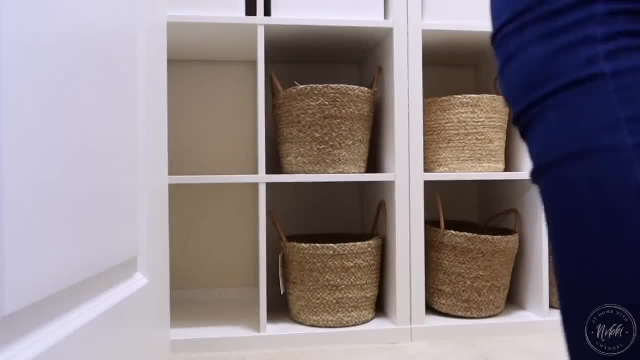 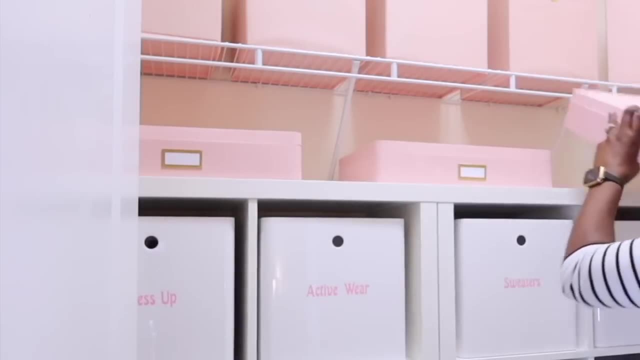 helpful in the long run. And then also with the baskets, get something that's lightweight for the kids so that they can really easily get into their basket and bring it and take the things in and out. And friends for the cube shelving in here. I got these from Ikea. They're very affordable. 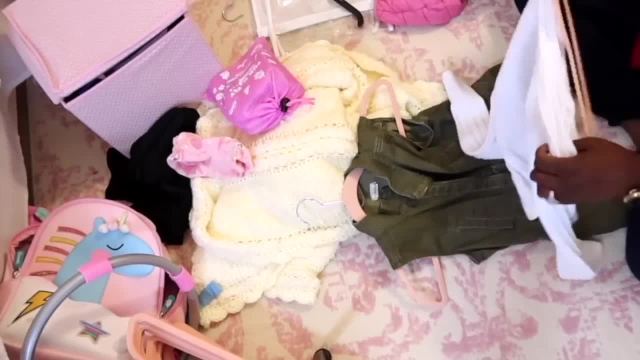 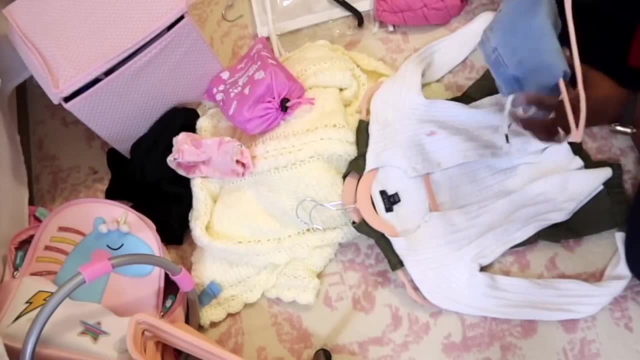 very durable, great for organizing a kid's closet or even toys and things like that. So now it's about dealing with the stuff and really paring down all of the things that she did not use or play with, which was a good bit, And that's what happens with the closet is. 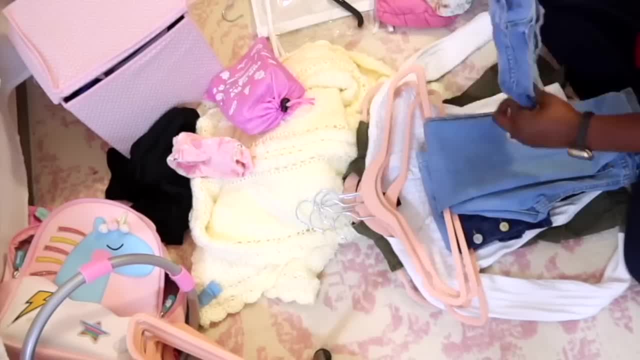 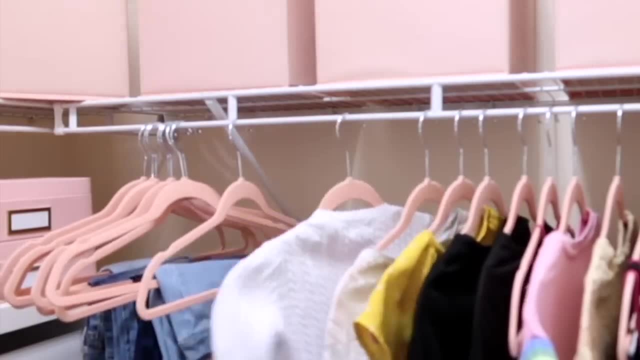 a black hole, a place to just tuck things And a lot of the things the kids have outgrown or they really don't use. And then, with the hangers, it's about hanging those clothes that her mom wants to grab for her, those everyday go-to, those essentials that she wants to be able to grab and go. 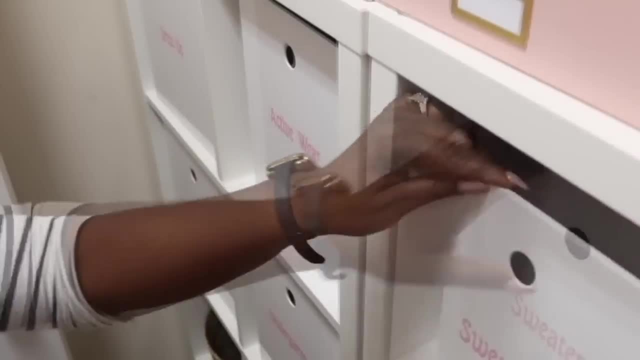 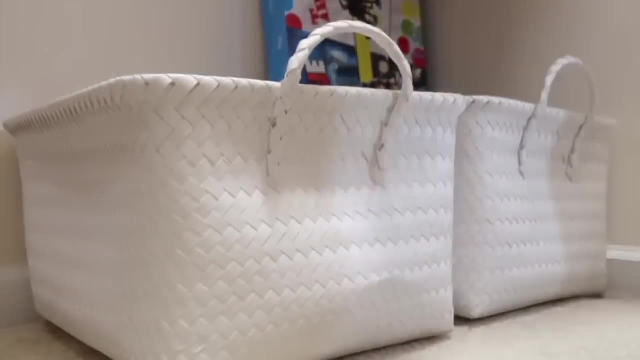 along with her coats and her sweaters and cardigans, And then in her bins are the clothes that are her everyday clothes, her play clothes, all of those things that she wants Savannah to be able to come and grab With the games. I'm going to stack them vertically, because this is 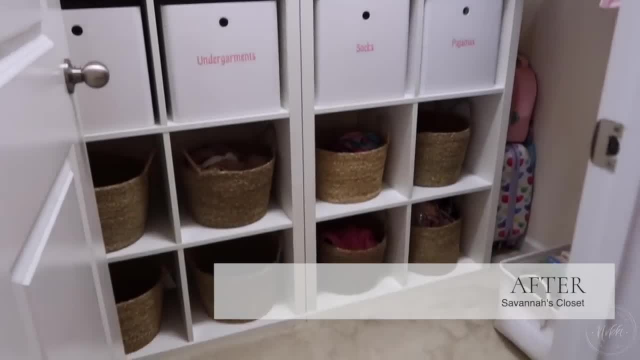 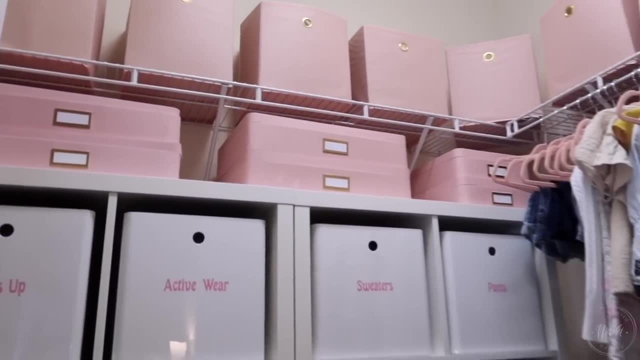 simple, but it makes it easy for her to get her games and to play with them. And then, with the closet, I'm going to put them back. They're on the floor, which makes it easy for her, but they're organized and efficient. So, friends, here is the closet, completed and now functions for a seven.